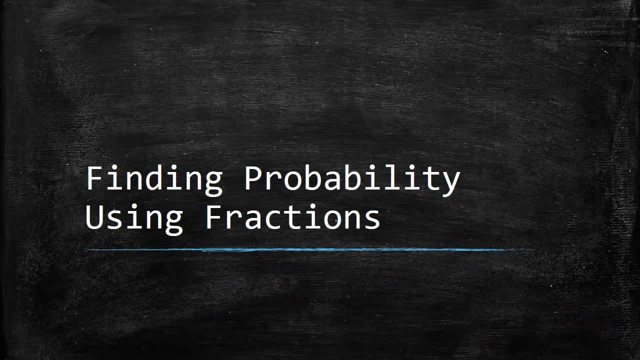 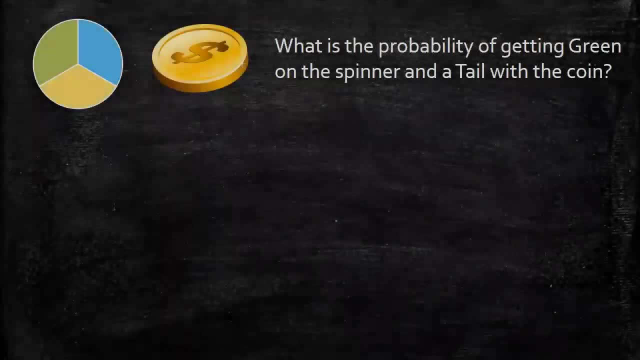 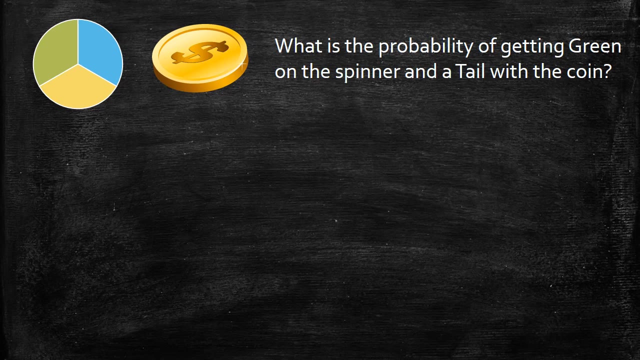 Here we're going to take a look at how we can find probability using our knowledge of fractions, and especially fractions multiplication. To start off, let's start with another example here. So we're going to look at finding what is the probability of getting green on the spinner. 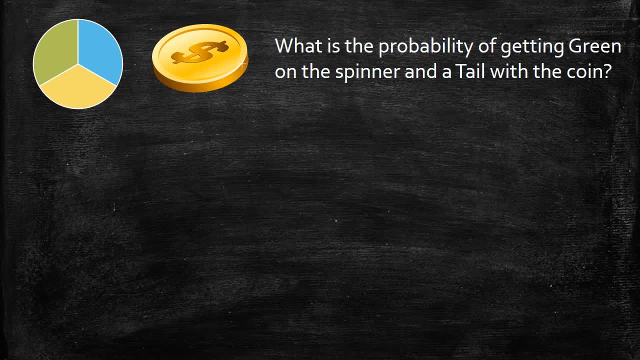 and a tail with a coin. So we know how to do this using a probability table. so that's what I'm going to set up first. So I'm going to set up my coins over here and I know that I can get a heads or a. 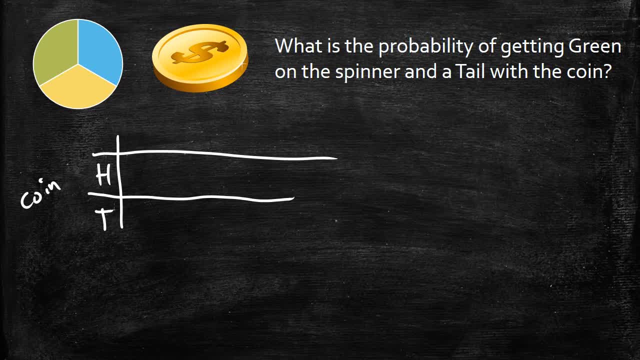 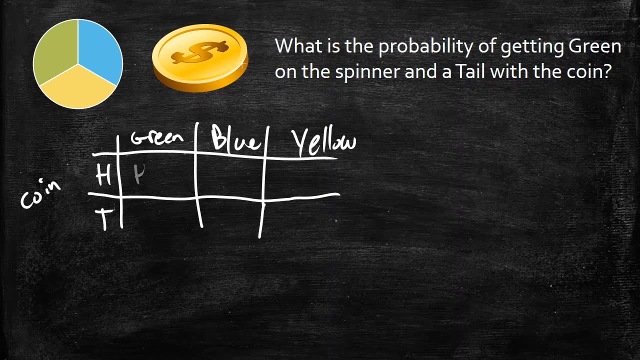 tails. Now I'm going to set up my spinner. I know that I can get a green, a blue or a yellow, and I'll just straighten out my table here a little bit. If I start to look at my results, I can get a. 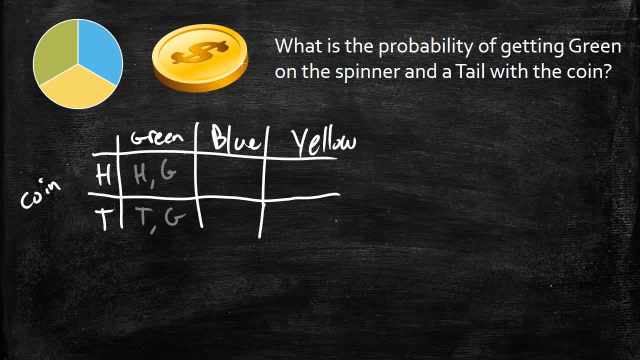 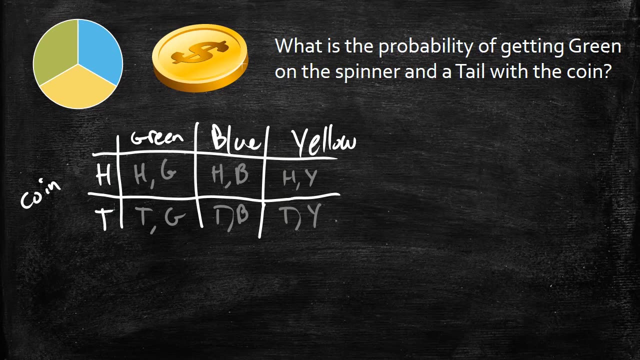 head or a green. I can get a tail or a green, get a head or a blue, a tail or a blue, a head with a yellow and a tail with a yellow. So just looking at this I can figure out really quickly just exactly my. 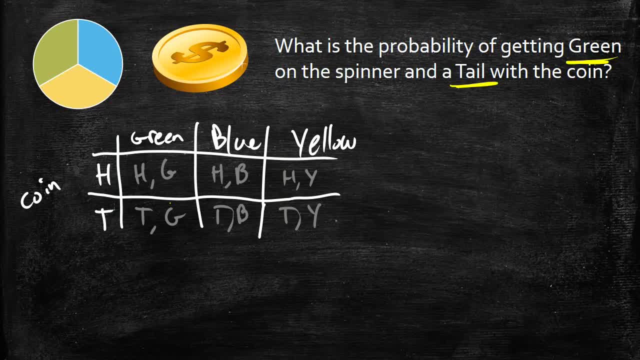 probability of getting a green and a tails, and I can see that right here: green tails and I know I've got it's a one and it's over a six here because I got six possible outcomes. But the other way we can do this and and we'll start with a very basic example- is by looking at the 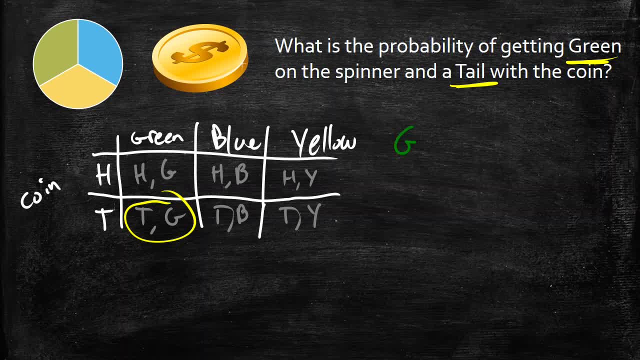 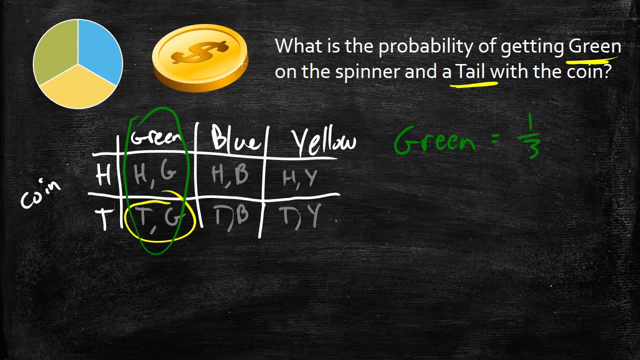 probability of each event happening on its own. So if I take a look at the probability of getting a green, I know that there is three options that I can get out of a spinner: a three-sided spinner with these colors, and I know that the probability of getting a green is one-third Alright. and then 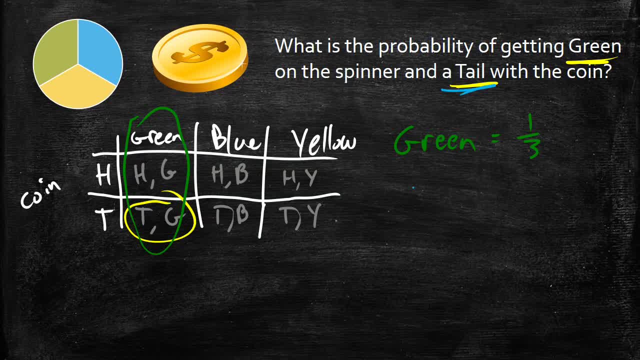 I can look at my coins, What's the probability of me getting a tail, and I know if I get a tail. there's only two possible outcomes: a heads or a tail. The tail is going to be one half of the options. Now the way that I can use this is I can use my knowledge from fractional multiplication. 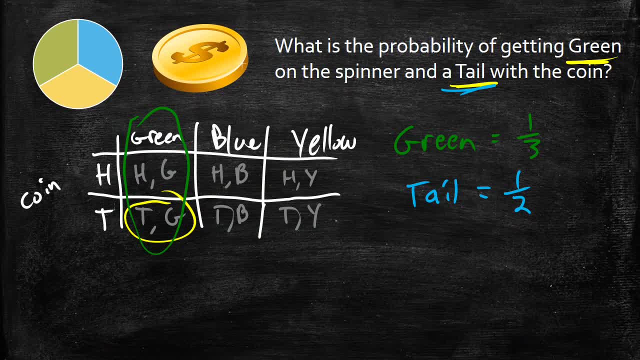 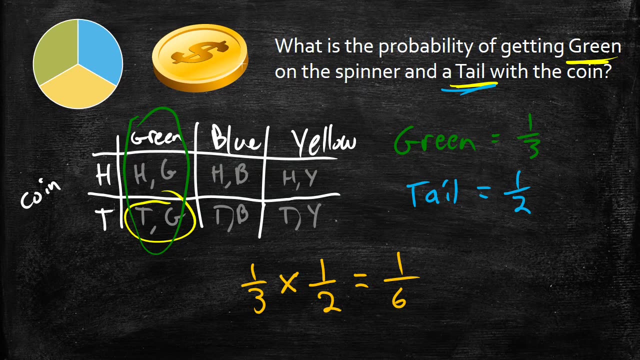 here and I can do my probability of getting my first outcome, which is green, and go one-third. I can multiply that by the probability of my second outcome, which is getting a tail, which is a half, and I will also. I will end up getting one sixth, because I know my top times, my tops, and my bottom times, my bottoms. 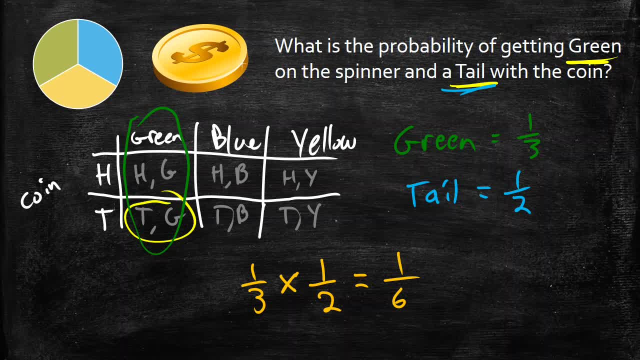 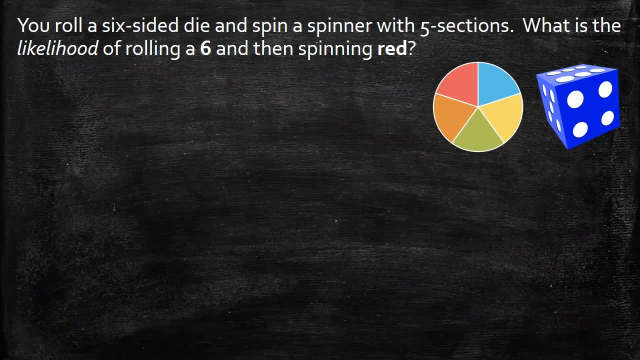 give me one sixth. So the probability of getting a green on the spinner and a tail with a coin is one sixth. Now we can kind of take this a little bit further and we can see where we can go with this. You're going to roll a six-sided dice or die sorry, and spin a spinner with five sections. 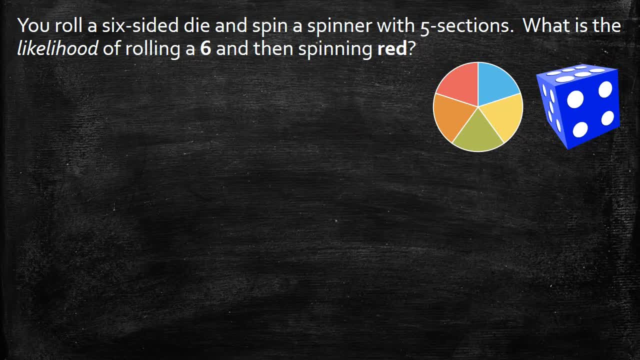 on it. What is the likelihood of rolling a six and then spinning a red? So I use the word likelihood here because that's just synonymous or means the exact same thing as probability when we see it in a question. So I want to take a look at what is the probability of rolling a six. So, rolling a six. 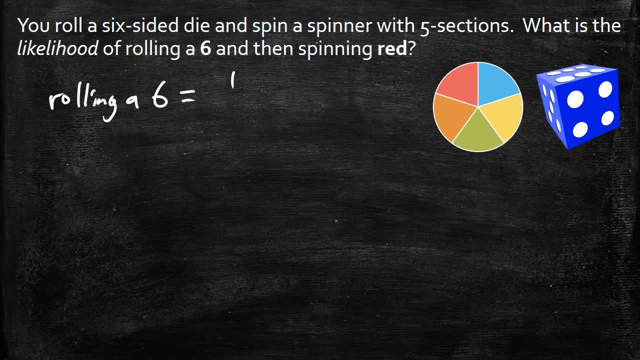 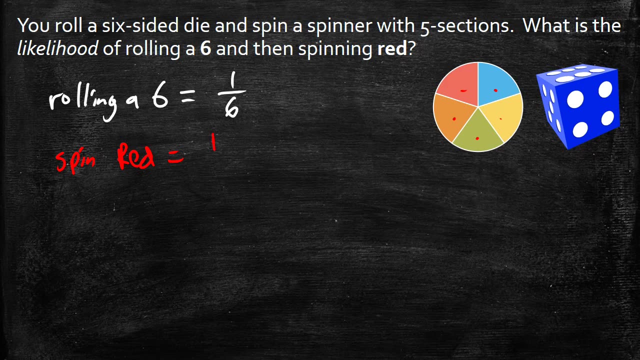 I know the probability of rolling a six is just going to be one, One out of six- because there's six possible outcomes. One of those outcomes is a six. Okay, I'm spinning red, Spinning red. There are one, two, three, four, five options. One of them is red. so 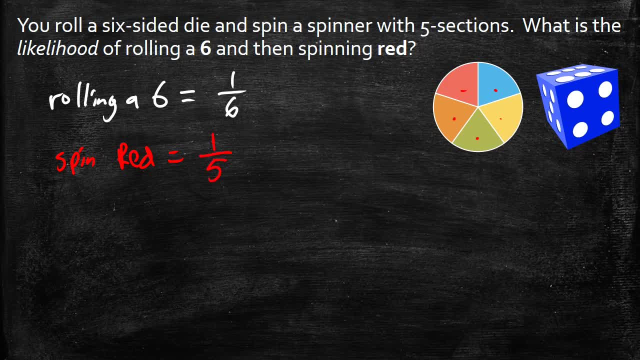 I know I have one out of five options gives me the probability of spinning a red. Now, just like we saw in the previous section here, to find the probability of doing both of these, I can just multiply these together. So I can go my probability of rolling a six, which is one sixth times the 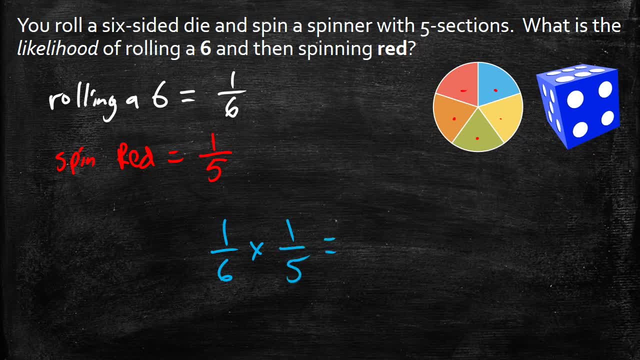 probability of spinning a red, which is one sixth. So I can just go one out of five options. So I can: fifth and multiply these guys together 1 times 1 is going to give me a 1 over a 6 times a 5, which gives me a 30. so my probability here is 1 out of 30 or we. 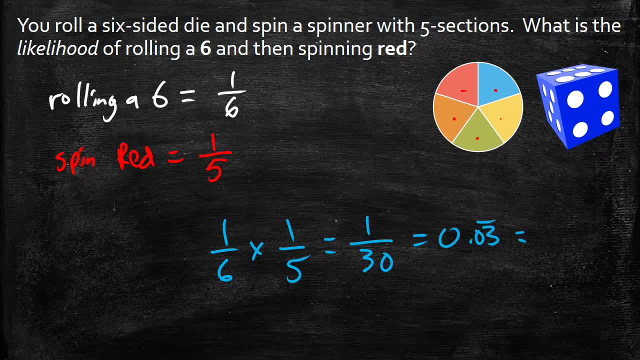 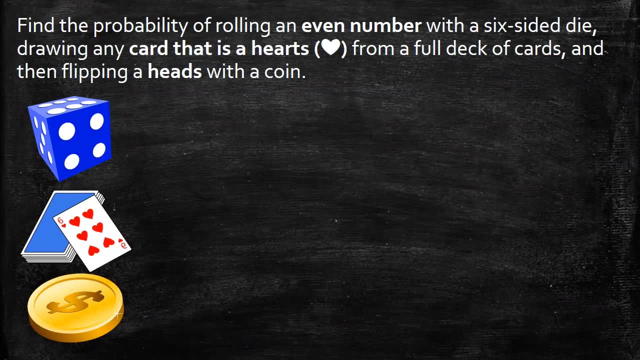 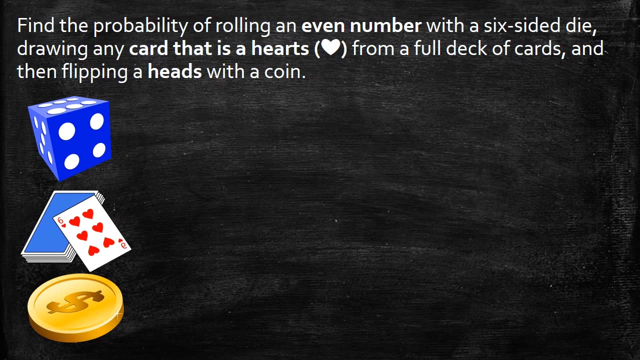 can write that as 0.03 repeating, or we can write that as 3.3 repeating percent. now you take this a little bit further. we can look at events with 3 or more. you could even do up to 100. you could do as many as you want events, as long as they. 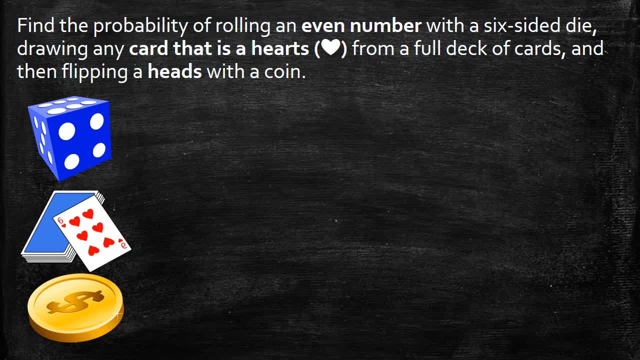 are independent events, events that don't matter to each other. so we're gonna look at this example. we're gonna find the probability of rolling an even number on a six-sided die, drawing any card that is, a heart from a full deck of cards and then flipping a heads with a coin. so I'm gonna start by finding the 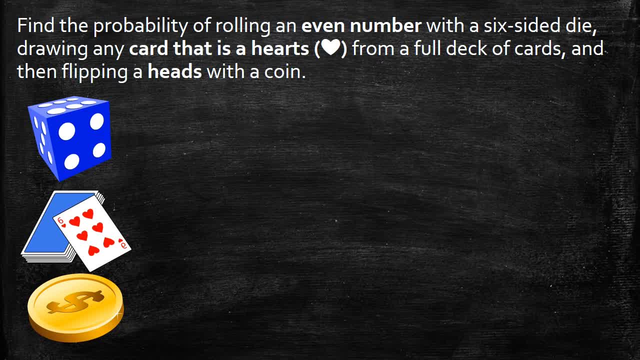 the probability of each individually. so I know I can roll an even number. so that's a two, a four or a six, that's three out of the possible six outcomes when we roll a dice. and I'm gonna simplify that, I'm gonna put that down into: